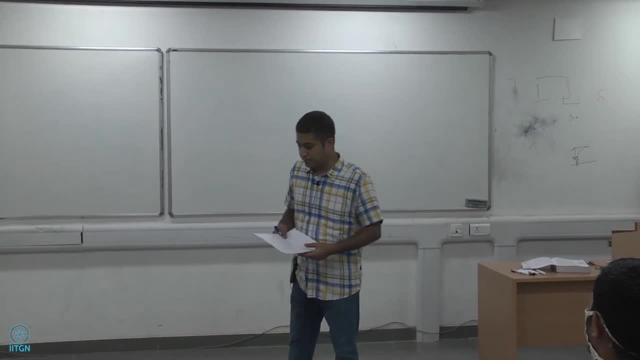 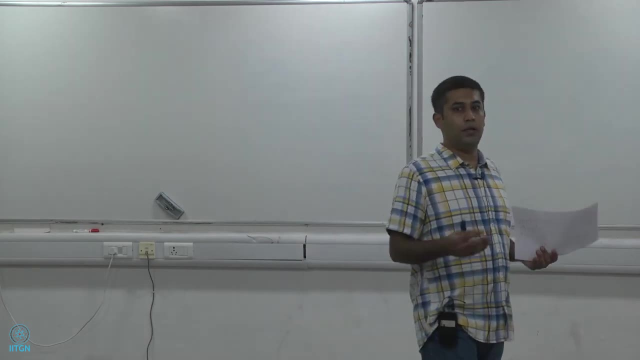 So that is why it is important to get a feel for units right Today we are going to this lecture. we are going to talk about something equally important, something very fundamental, and that is systems and the future of the future. 1. 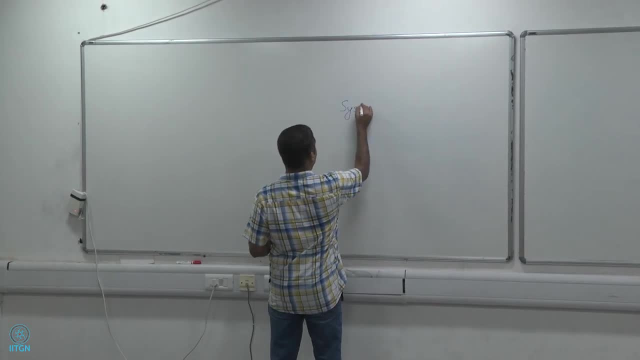 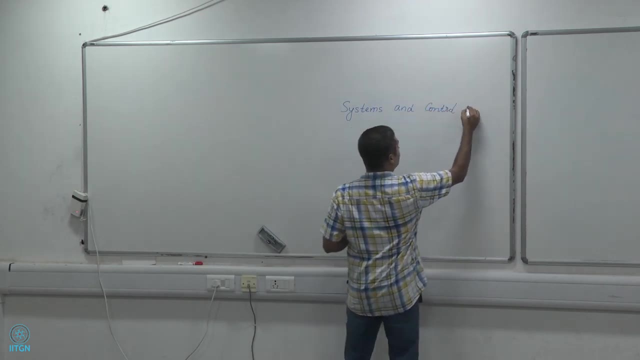 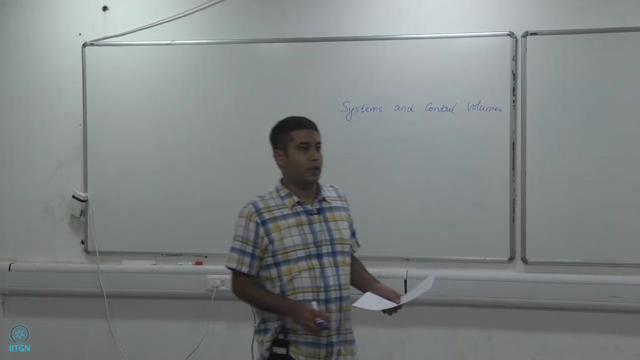 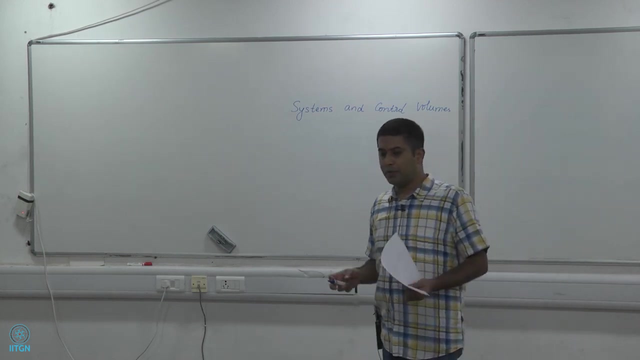 and control volumes. Now, when I actually talk about what a system is or what a control volume is, you will feel: how is this fundamental? this is very simple, right? This is perhaps the simplest thing of all. it is just a box, at the end of the day, which. 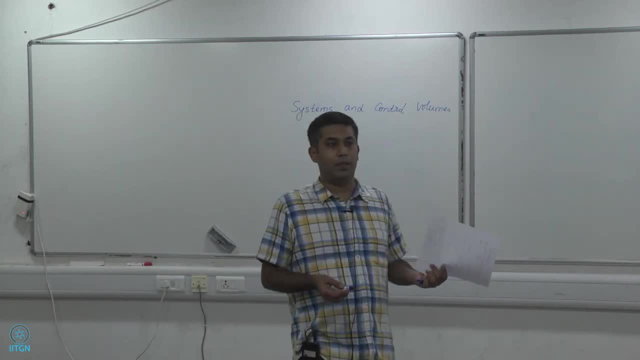 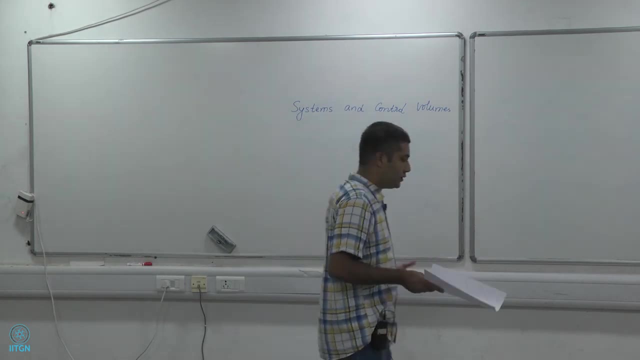 is a box, you call it a system, you call it a control volume. what is the big deal? right? and yet this is the biggest deal. sometimes, and you will not believe me when I say that many faculty candidates who come to IIT Gandhinagar after their PhDs, or many times after their 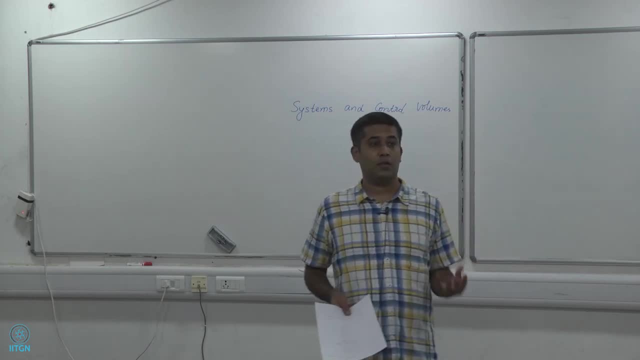 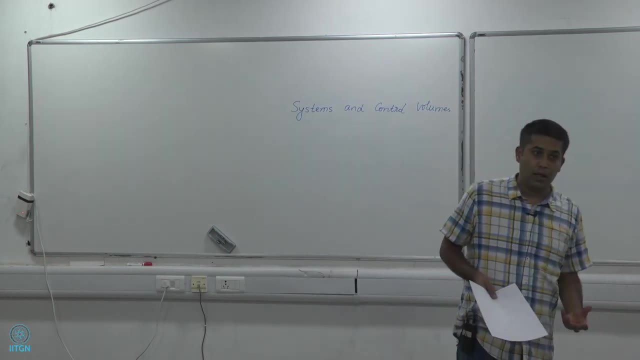 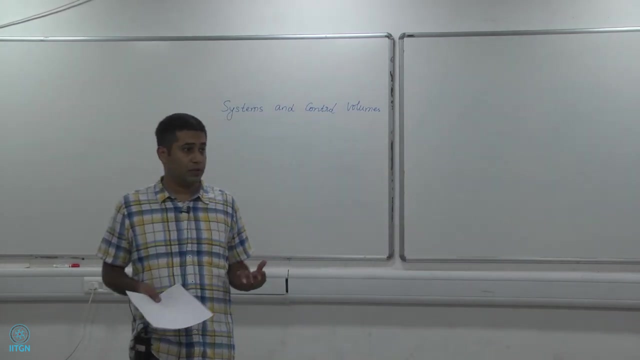 post docs are not able to draw systems and control volumes correctly, and that is because they think it is too trivial and they ignore it and then it comes back and bites them. So it is very important to understand what a system or a control volume is and it is. 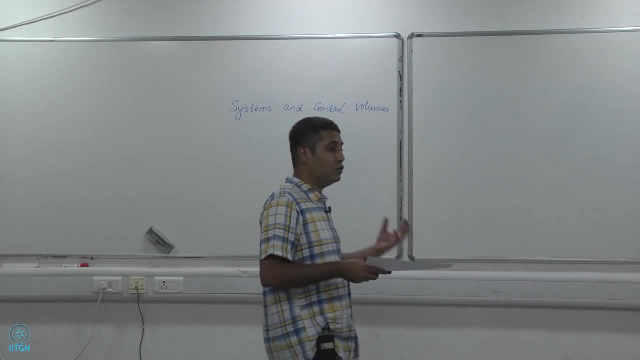 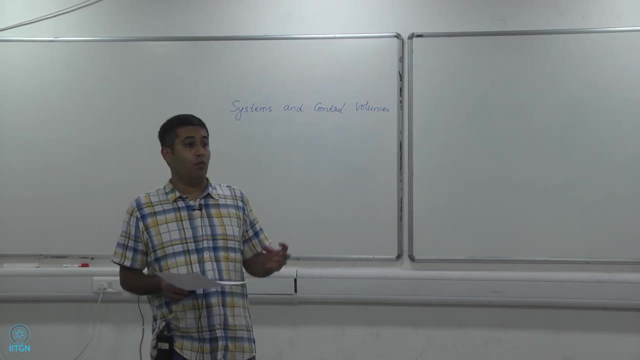 important to understand which control volume or which system to use when. and it is also important to understand, once we draw a system or a control volume, what is inside the volume or the system and what is not inside the system or the volume, and it is very important to 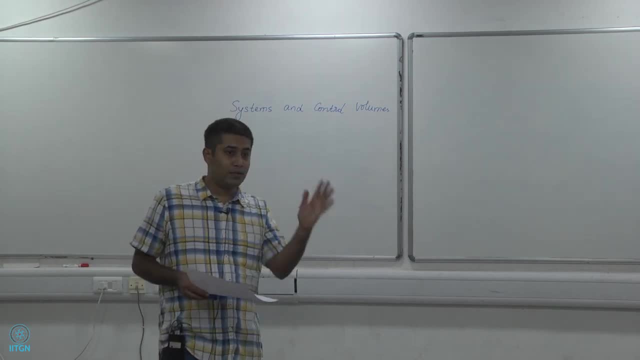 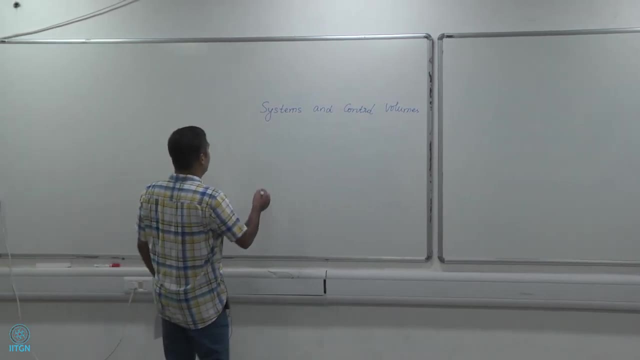 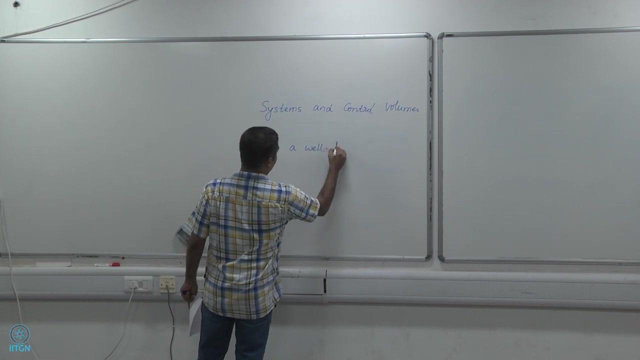 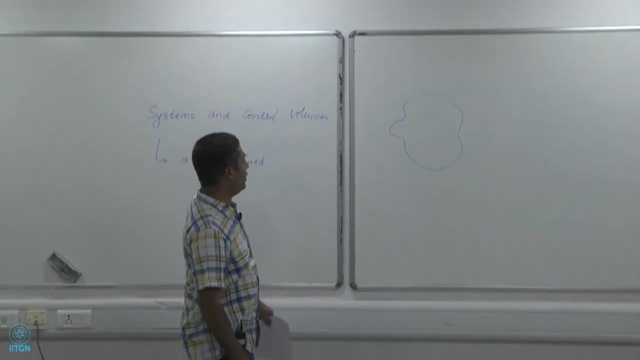 have that clarity. where is my boundary? what is inside and what is not inside? Okay, So what is the system? It is basically a well defined mass, So it is basically. it could be any shape. So, for example, I could have a system like this, and there is something. 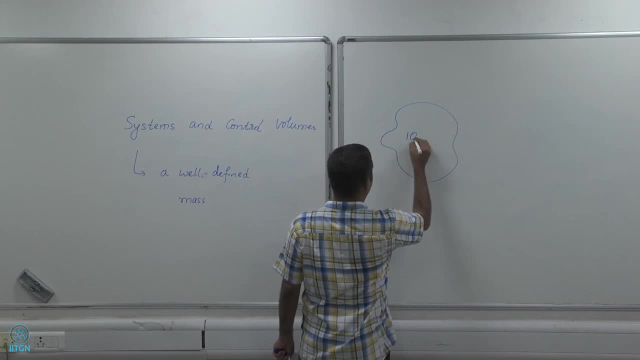 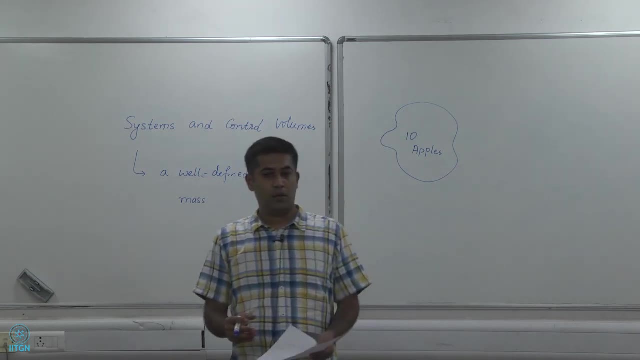 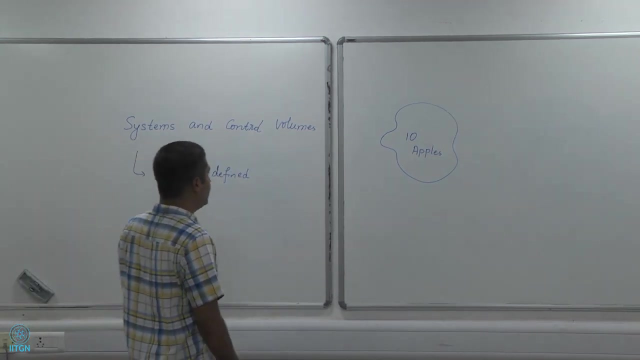 inside. Let us say there is 10 apples inside, So I could have a system that includes those 10 apples. Now, what is important about this system is that. So these 10 apples remain 10 apples. The mass of a system does not change. So no apples. 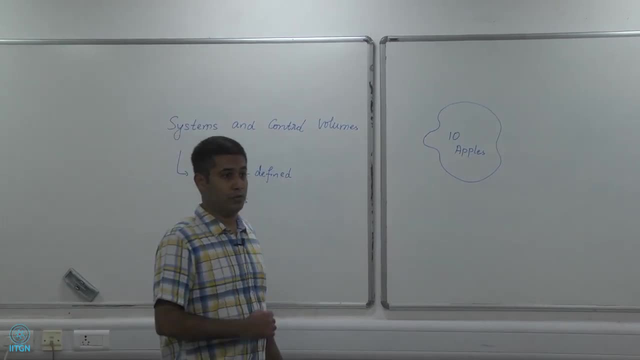 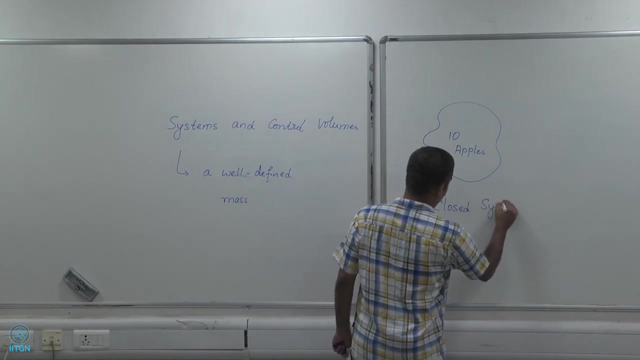 can be added to the system and no apples can be removed from the system. So if you do that, then it no longer is a system. It becomes something else which we will discuss later. So it is a closed system. It can be called a closed system or just a. 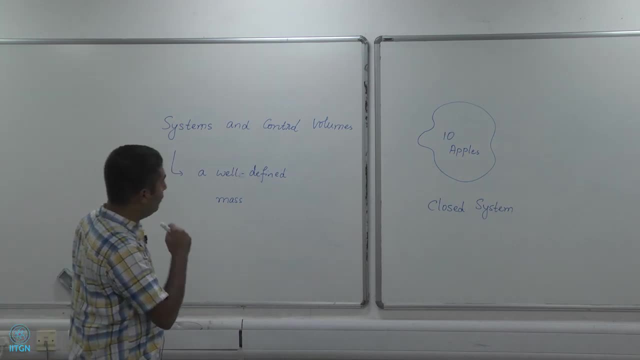 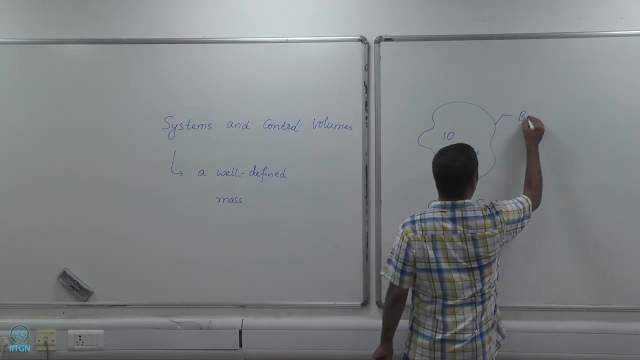 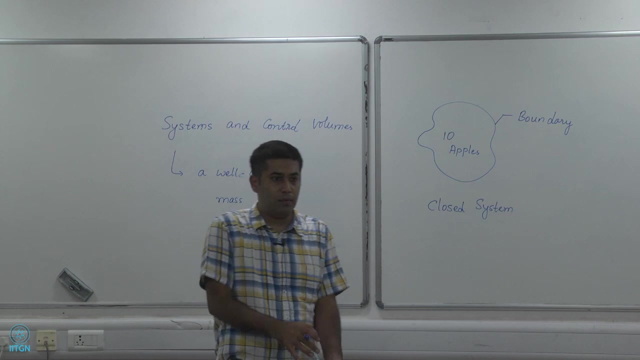 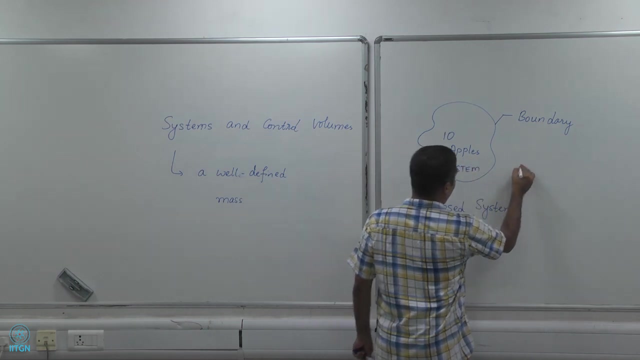 system. Well, basically, these things are always in the system, And what does this also have? This is, as I said, a fixed mass system and there is a boundary, And the boundary separates the system from the surroundings. So this is the system And this is the surroundings. 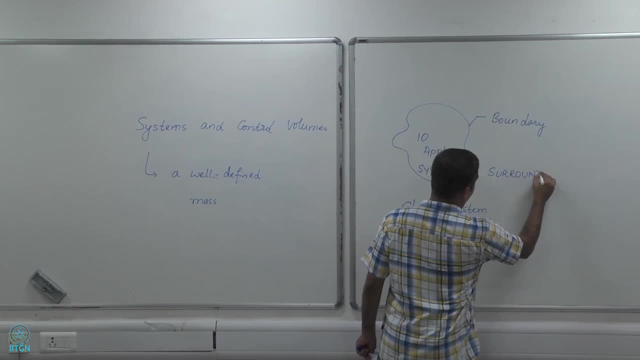 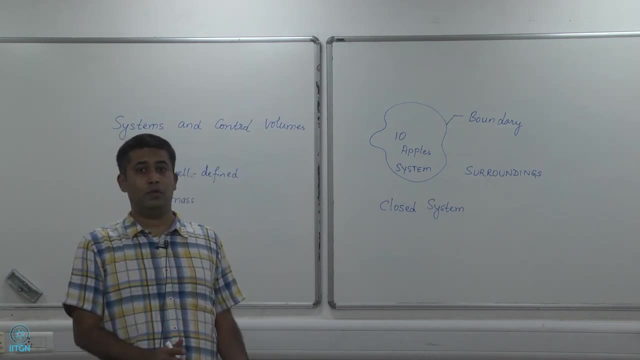 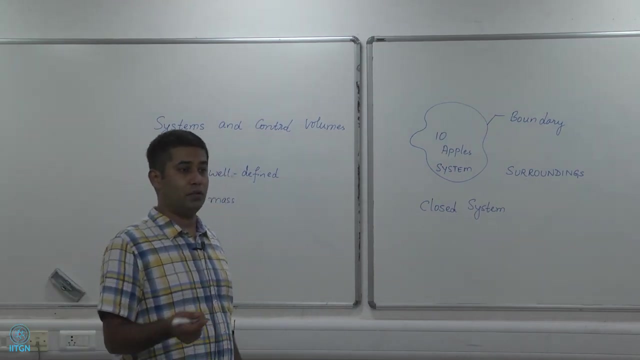 Right, hadi Kalai. So a well-defined boundary separates the system from the surroundings. Now, what is the thickness of the boundary? How thick is the boundary? It is not. it is extremely small, negligible. it begins. 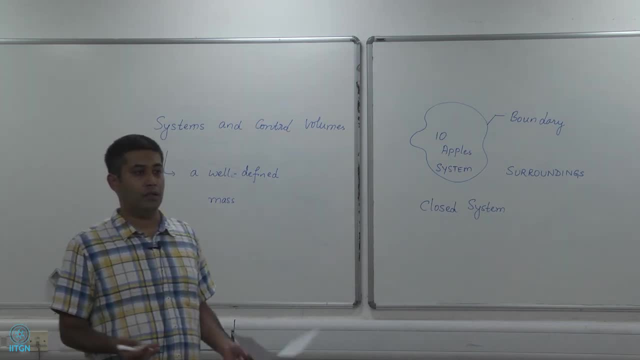 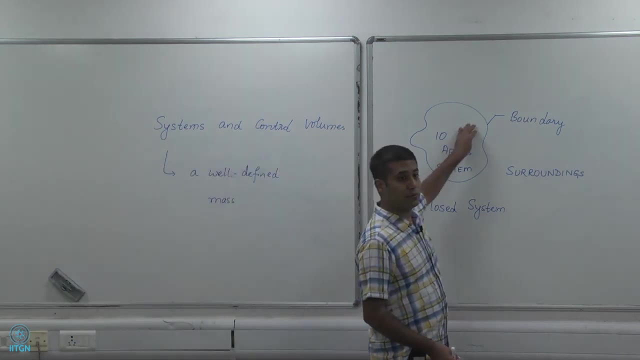 Right, Mathematically it is infinitesimally thin, so it has zero thickness, and yet it separates the system from the surroundings. Now you might think again: what is so? what is the big deal about this? So let us think about the human body. 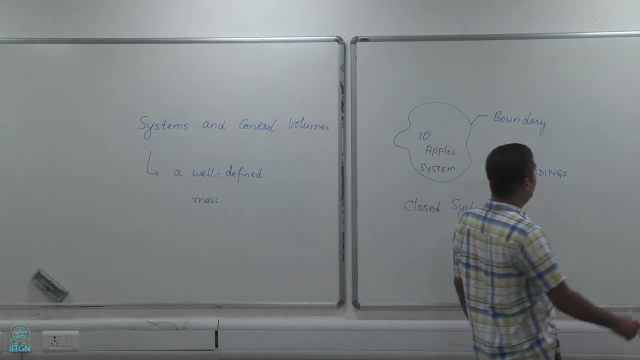 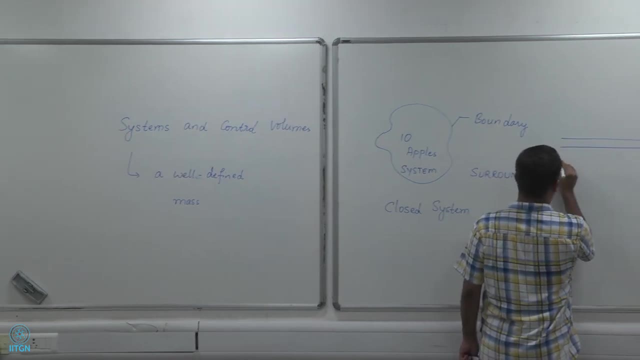 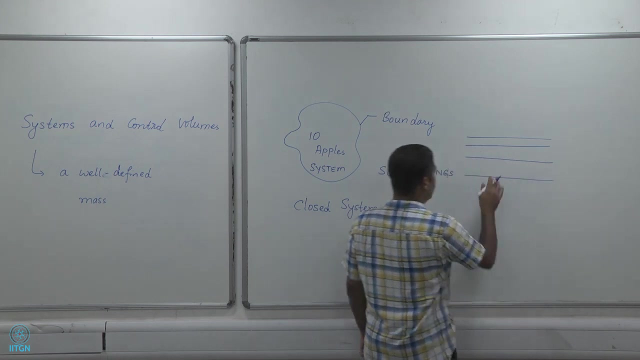 Right, Let us think about the skin, for example. So if you look at the skin, if you look under the skin, so that is the outer skin layer. perhaps there is a fat layer, perhaps there is other things inside, So let us say there is a muscle inside. 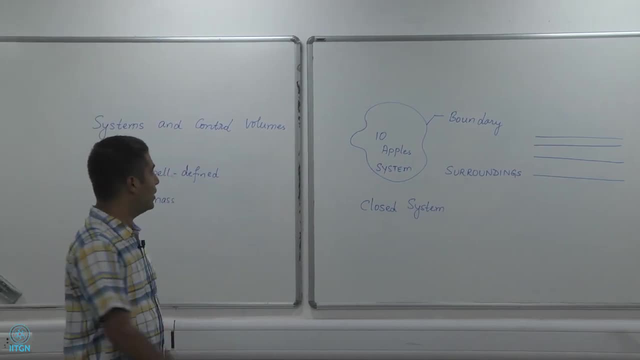 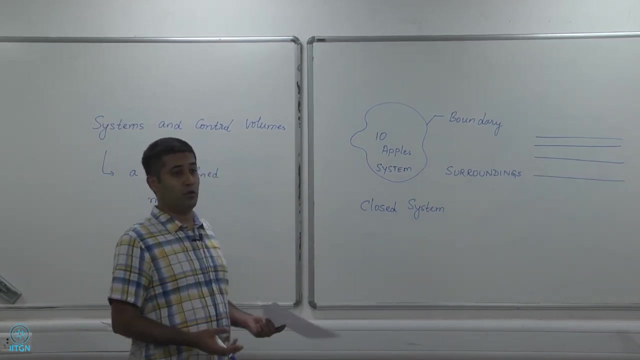 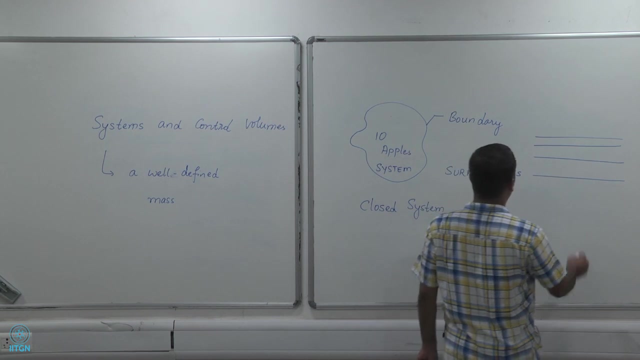 And there is a fat layer out on the in the middle, and then there is the outer skin Right, And let us say that you are trying to analyze energy transfer from the, from the skin, to the outside Right, And let us say that you take a system that looks like this: 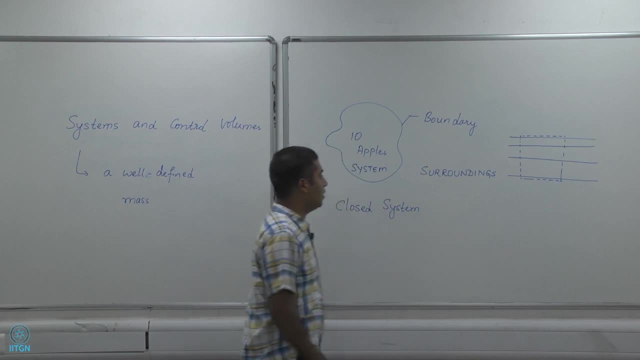 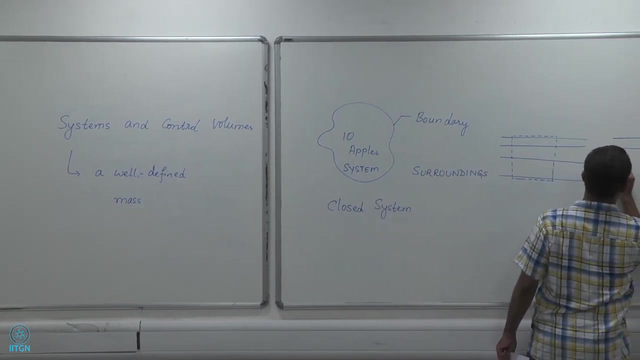 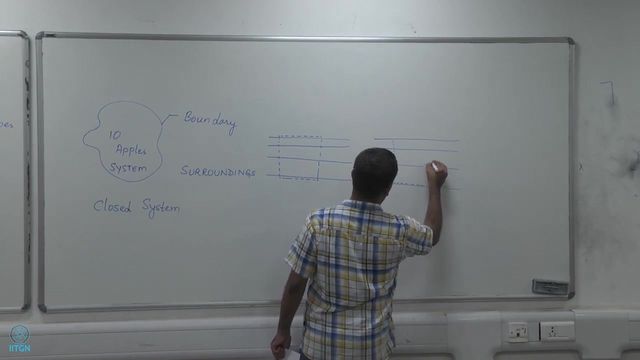 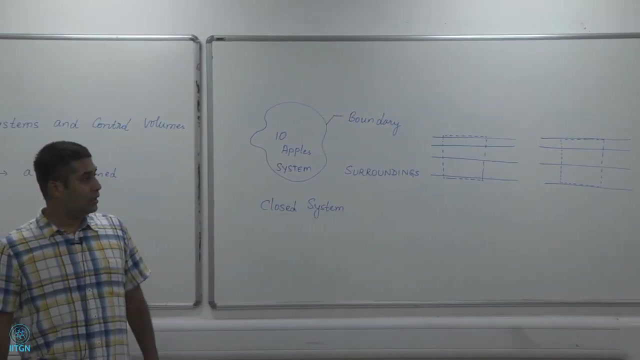 Right. And let us say: that is your system. you call that your system. So, and then the same situation. let us say that you have another situation in which your system is that: Now do you think physically, Do you think? 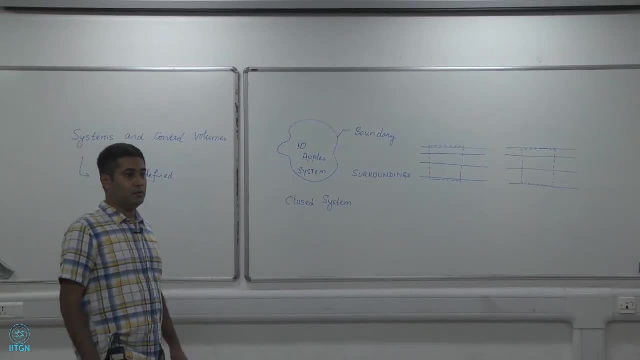 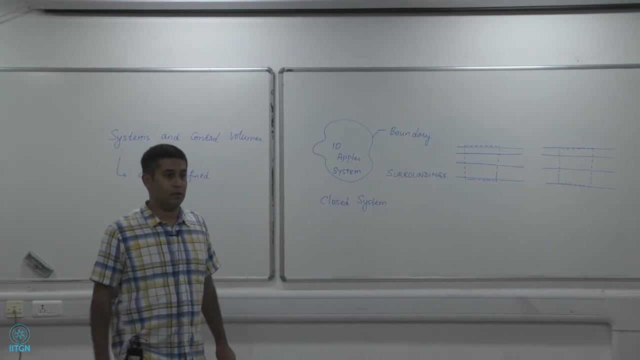 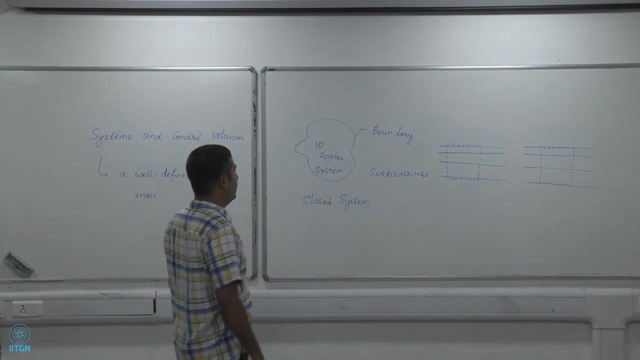 Yes, The size of those two systems is different. No, It looks similar, It is the same. The size of those two systems is the same, But yet are those two systems different? Why are they different? In second one, you have not considered the outer layer, like which is: 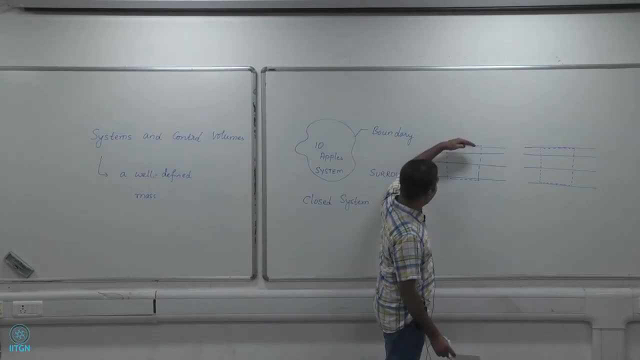 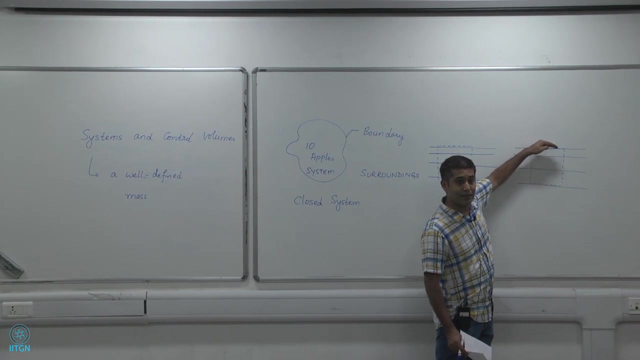 Right. In this, the system boundary is such that the outer surface of the skin is inside the system boundary. In this, the system boundary is such that the outer skin, the outer surface of the skin, is not inside the system boundary. So what? 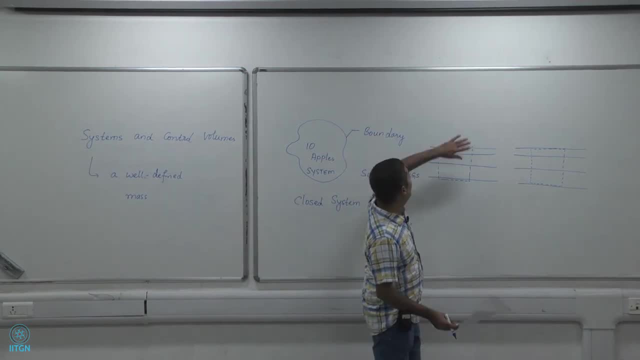 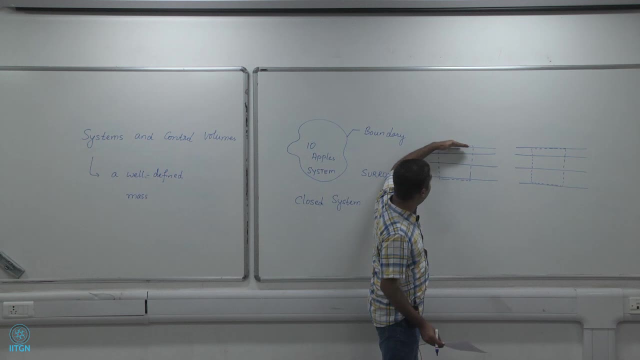 So what happens? So what happens is that let us say you have the room or the air or something outside. Here you have got to consider the heat transfer from the outer surface of the skin to whatever is outside Right- Air, you know, room, whatever. 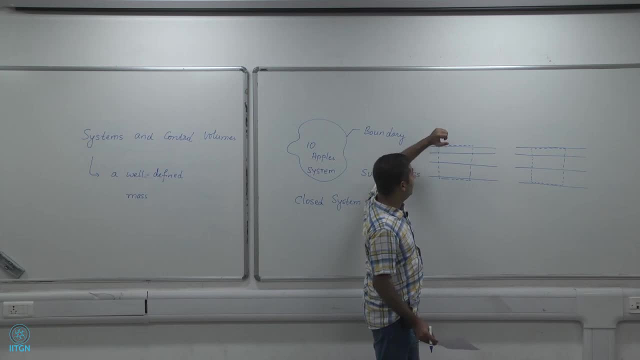 Right, Other people here. yes, you have got to consider that, but then it is only a different kind of heat transfer Here. if it is a solid, this is a conductive heat transfer because this boundary is inside a solid. Here, this boundary is actually in a fluid. 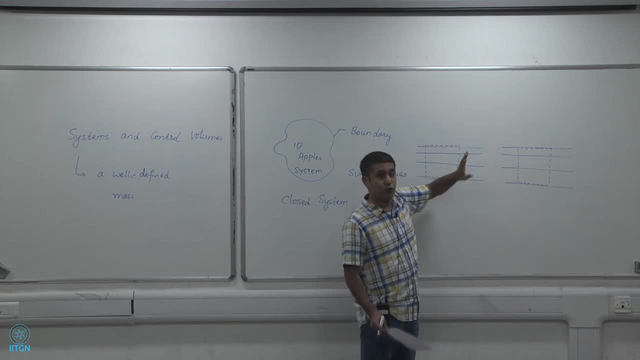 Right. So there it is, a different kind of heat transfer, Right, Those two heat transfer might ultimately be equal, but at the same time, you must recognize that they are different. They are different in the sense that they do not include or include the outer surface. 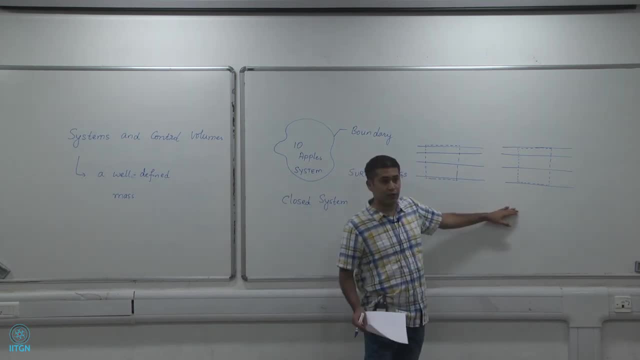 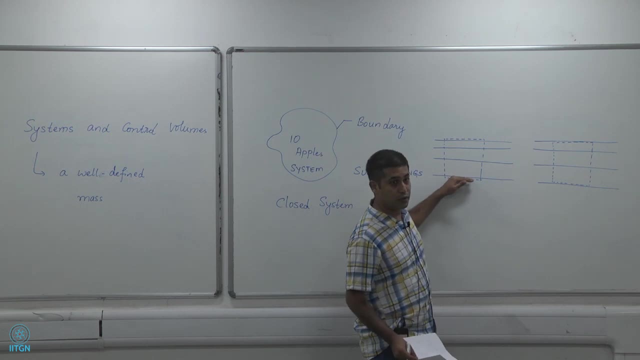 of the skin. Similarly, let us say: there is a blood vessel here, There is a blood flowing here. Right, I have got to consider here the heat transfer between the blood and the outer, the inner surface of this, whatever this muscle is. 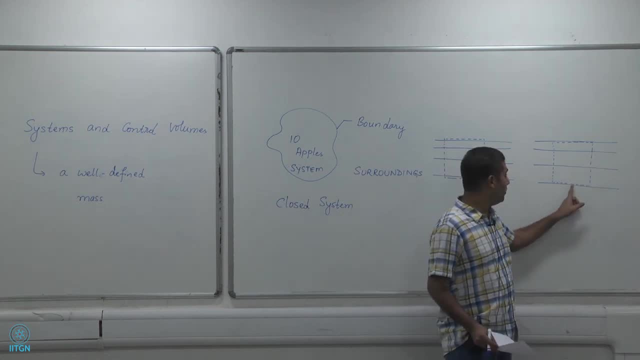 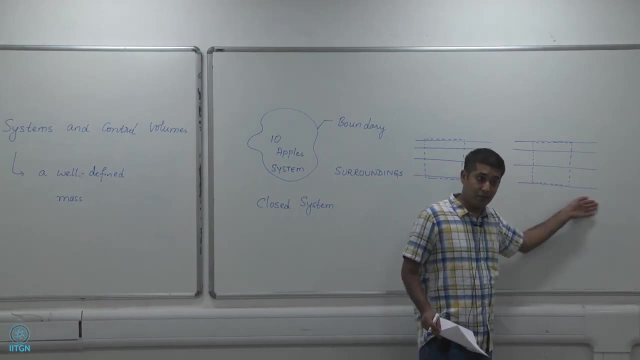 Right Here I do not. Okay, It does not mean there is no heat transfer here. There can be heat transfer, but I do not need to worry about the temperature of the fluid that is flowing here to consider Right This heat transfer. 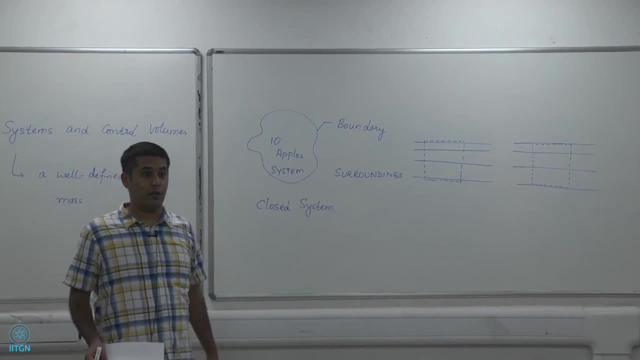 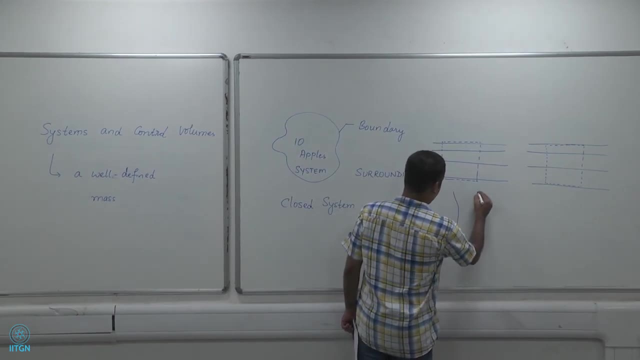 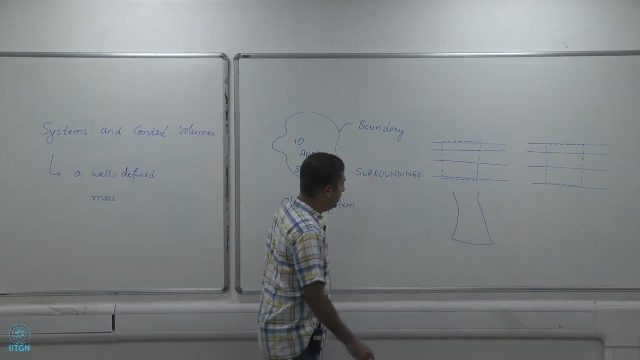 Right, So I just need to consider the temperature of that surface there. Okay, So similarly, for example, if you have a rocket engine, this is how the nozzle of a rocket engine looks like. Right, This is a converging, diverging nozzle. 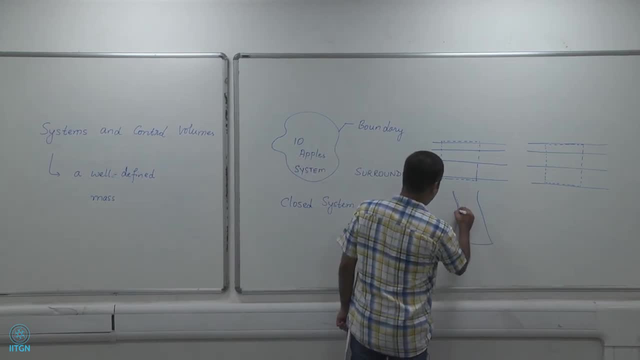 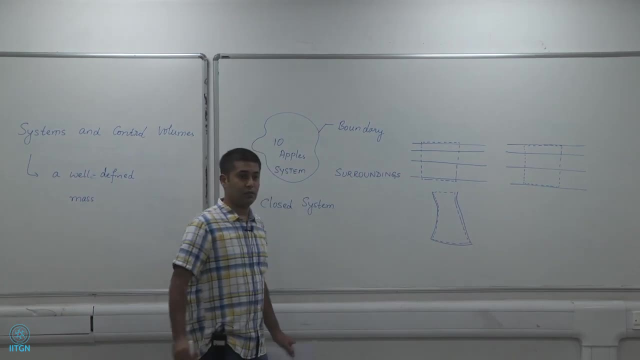 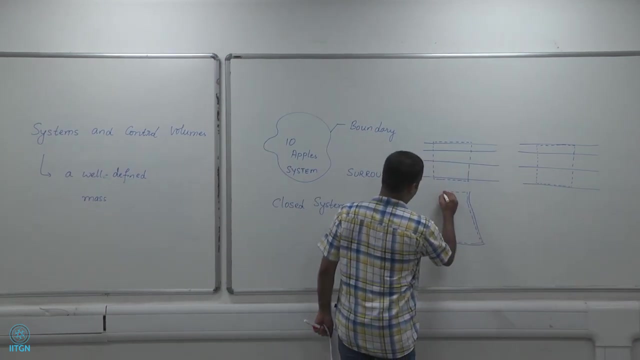 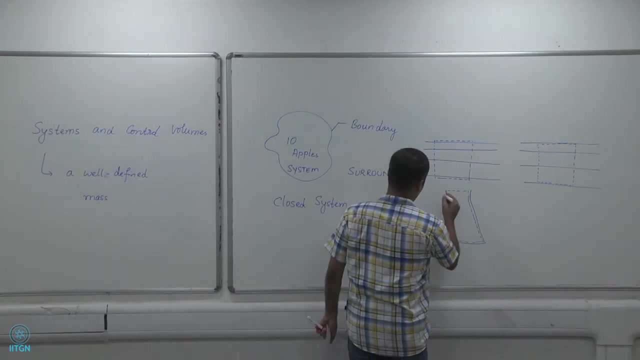 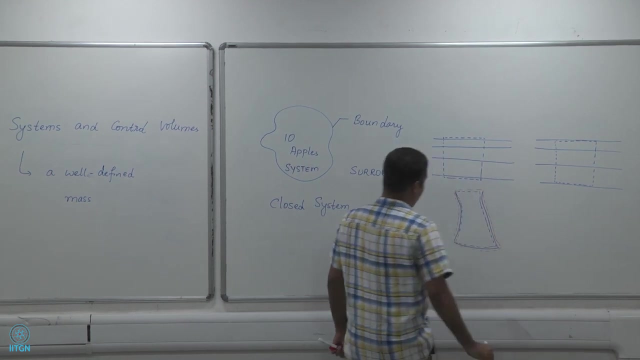 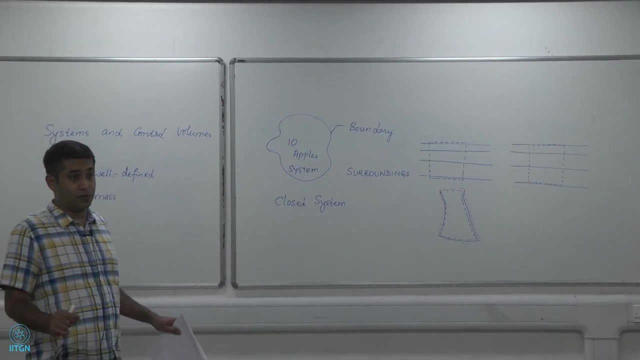 So if I consider the system to be Right, That Okay. So that is my system, Okay. And the other way is to consider my system to be The blue and the red systems, although their sizes are exactly the same, or perhaps almost. 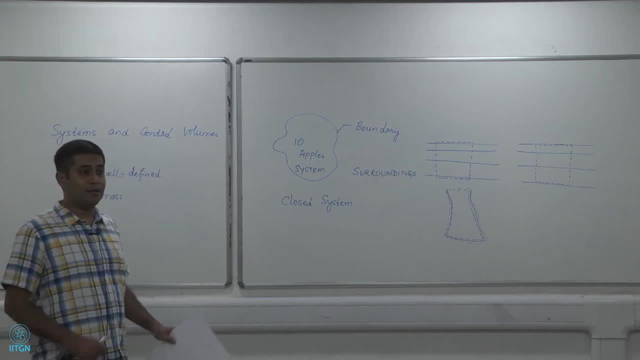 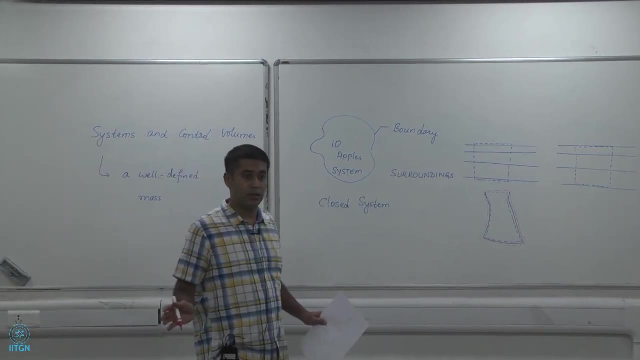 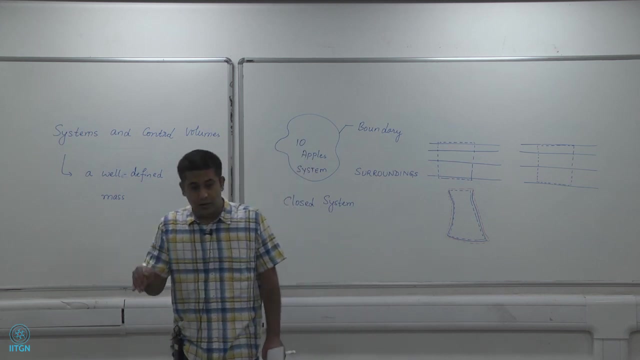 the same, Right. They are very different. Their energy interactions, the equations that I get when I write energy balances for those systems are very different, Right, And so it is important to know how to draw the system boundary. And once you have drawn the system boundary, it is also important to know clearly what 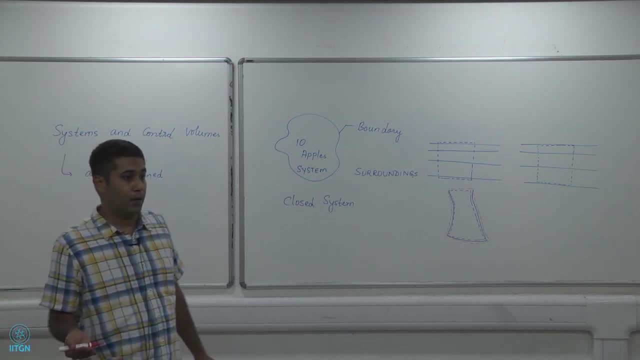 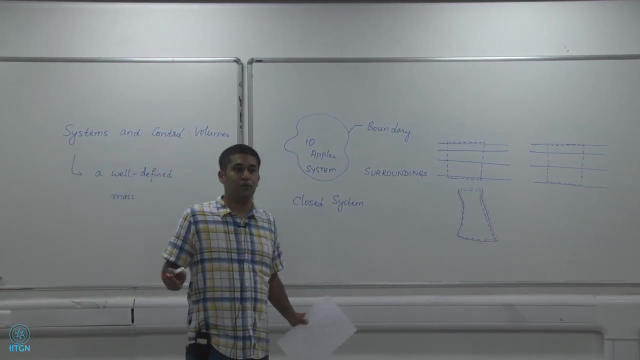 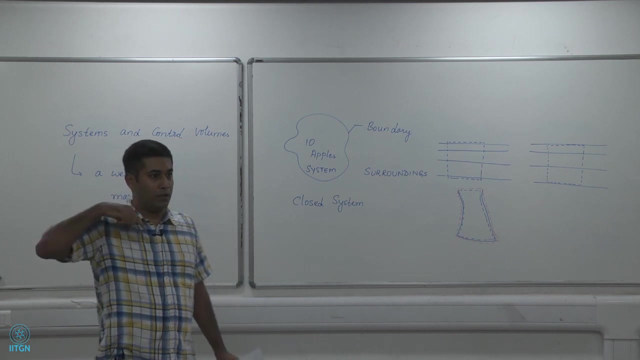 is inside and what is not inside, Okay, And what happens is normally we think a problem is so easy, We think a problem is so easy that we do not draw the system boundary And we have something in mind as to what the system boundary is or what the system is. but 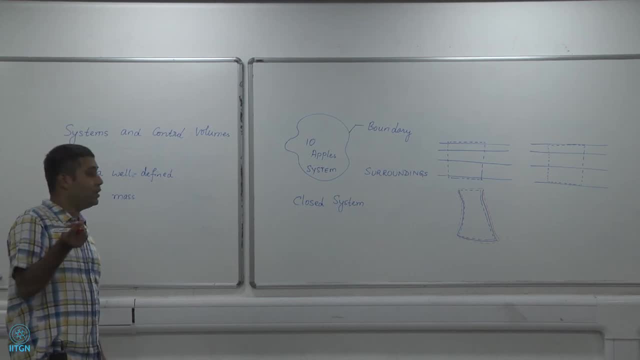 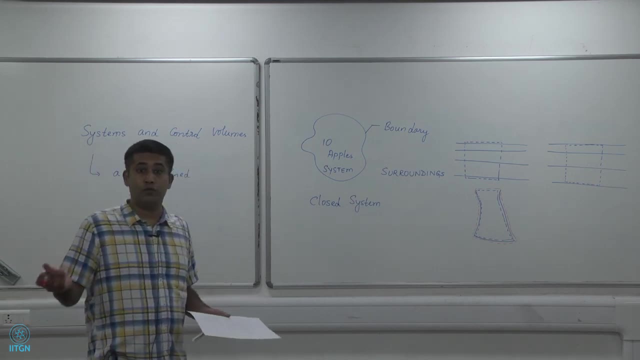 we write an equation for a system that we do not have in mind. In other words, we include some terms which we should not have included, or we exclude some terms which we should have included in the first place. Right, We make a mistake. 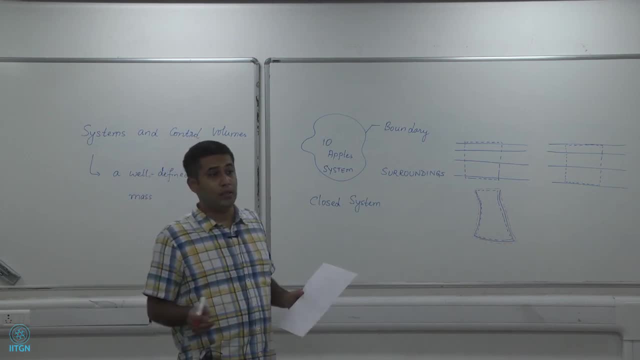 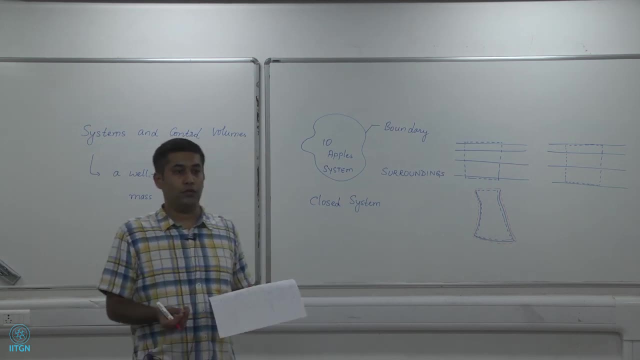 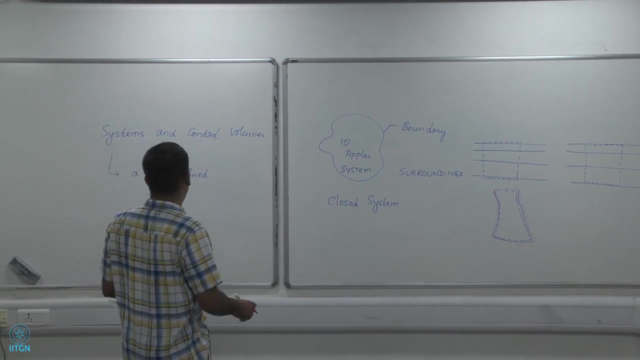 And this is done not just by undergraduate students, This is done by almost everyone who does not follow the simple procedure that you first have to define the system before you solve a thermodynamic problem. Okay, So it is very important to understand what systems are, what is inside and what is not. 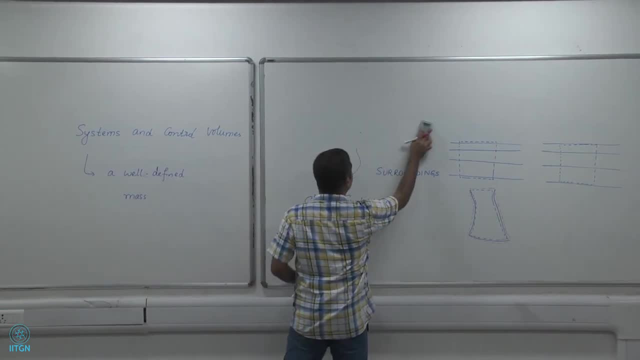 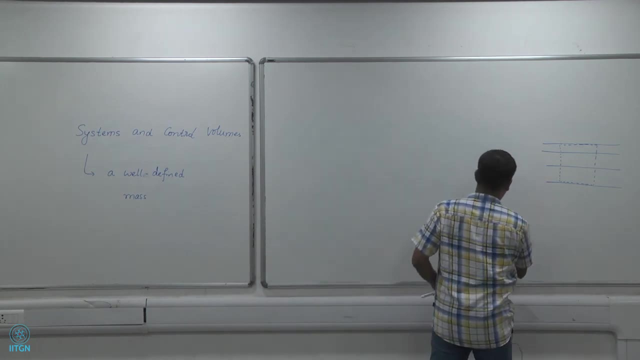 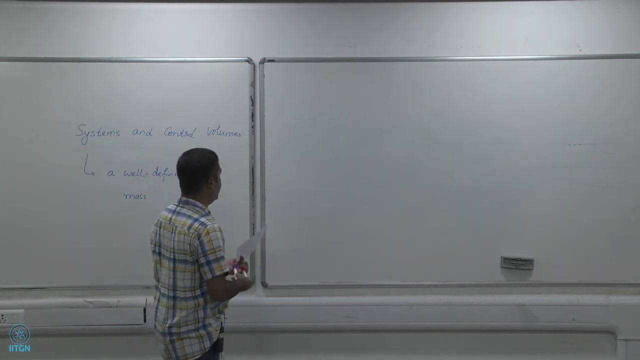 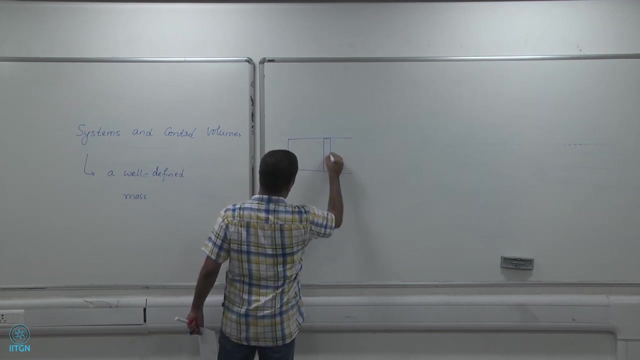 inside. Now, can a system change its volume? Yes, it can. So, for example, I have, let us say, a cylinder and I have a piston that basically traps some gas here. let us say air Right, And let us say this piston is movable and that it can move inside the cylinder, and yet 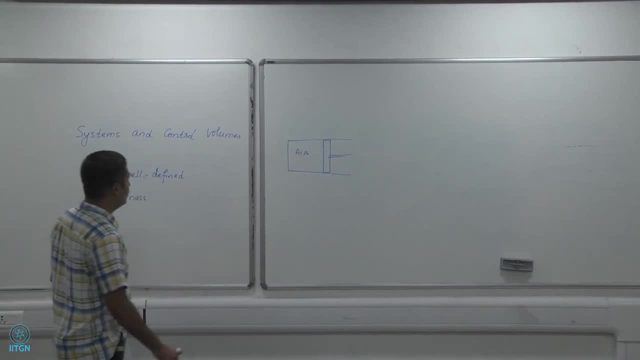 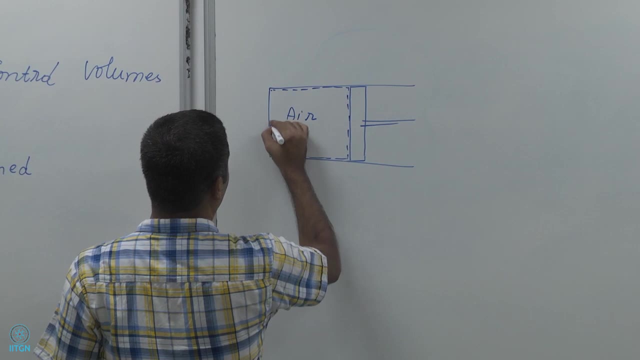 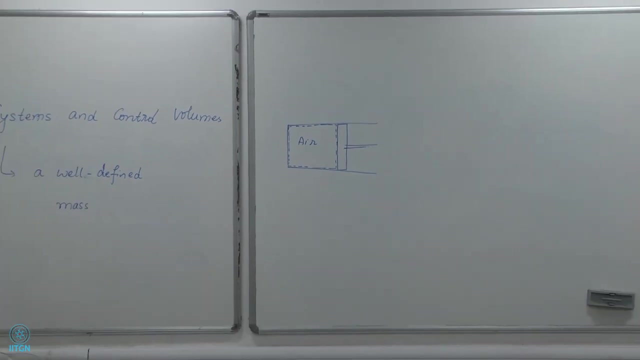 it is trapping some gas inside Right, And so I can consider this to be my system, Right. Why can I consider that to be my system? Because its mass is fixed, Although the piston can move and its volume can change, but its mass cannot change. 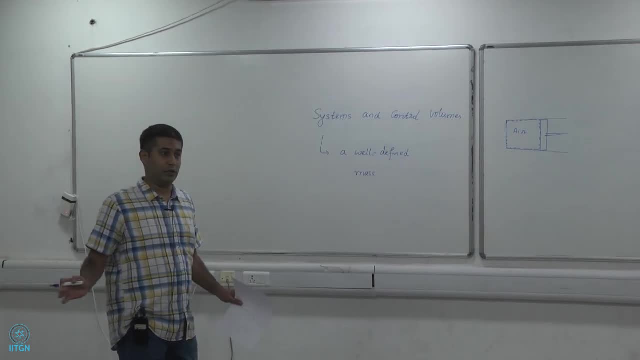 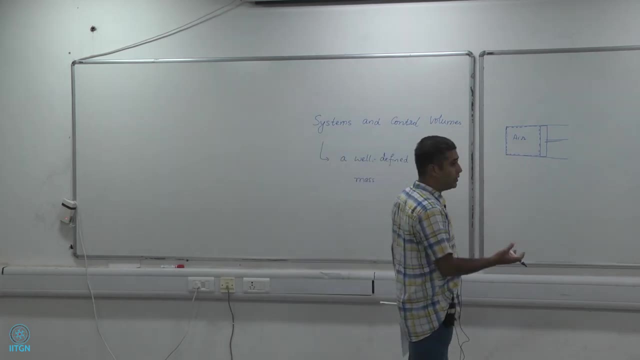 Right, So its boundary can move. I can have a moving boundary, That is okay, That is allowed, And but its mass cannot change. Right, I can have energy interactions. I can heat it up, I can cool it down. 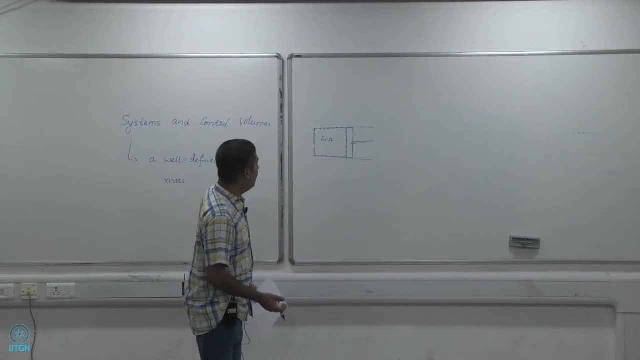 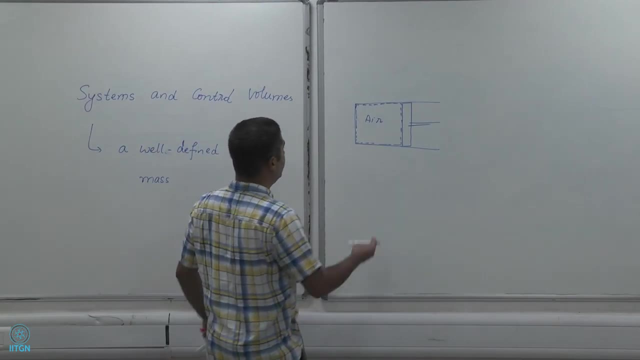 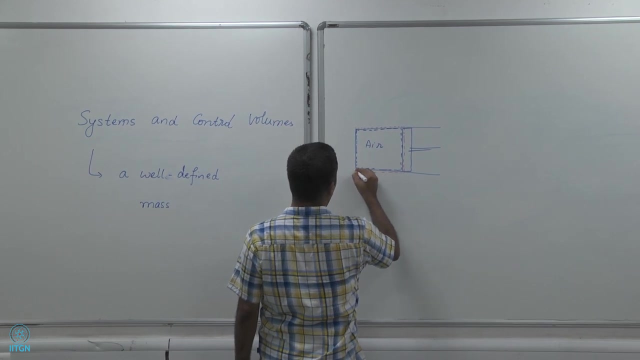 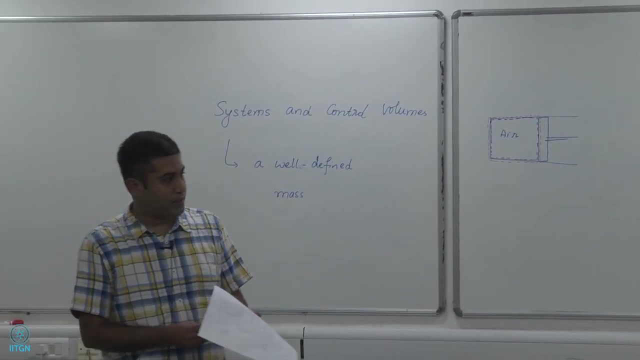 I can do other things to it, Right, But I cannot change its mass Right, And that is why it is a system. I can also define my system in this way. Right Again, if I do it like the blue dashed line, or if I do it like the red dashed line, the 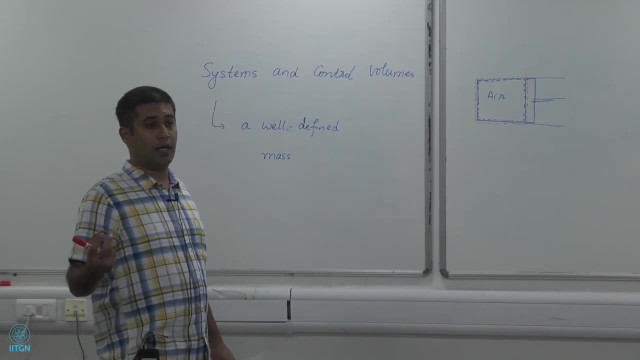 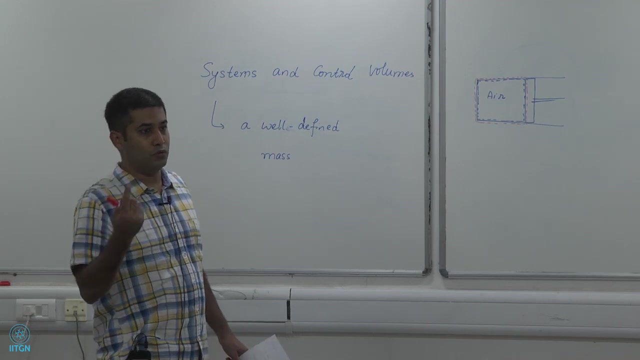 analysis is very different. Sometimes, the equations that I get are very different. Right, And if I have one mixed up with the other in my head, I am likely to do a mistake. Right, And it is very important, therefore, to pay attention to how you draw the system. 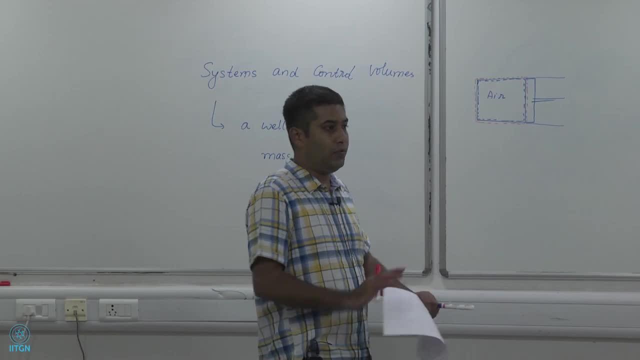 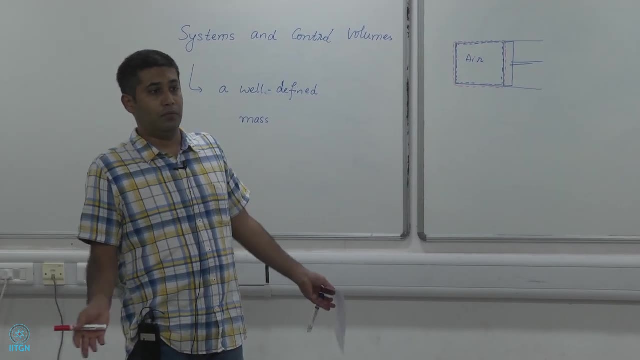 You can draw a system any way you like, Any way, Any way, Any system is allowed. You can have any system you like, But some systems help you to solve a problem. If you choose systems that are you know, for which you do not know some of the terms, 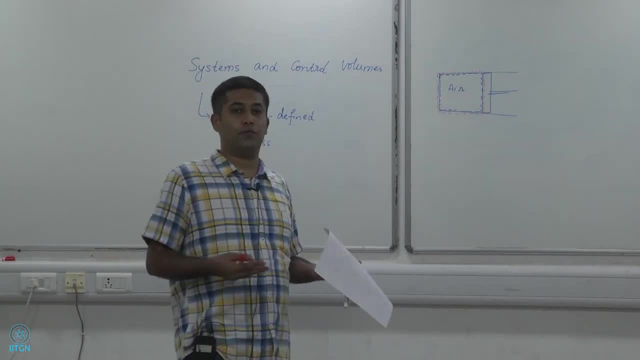 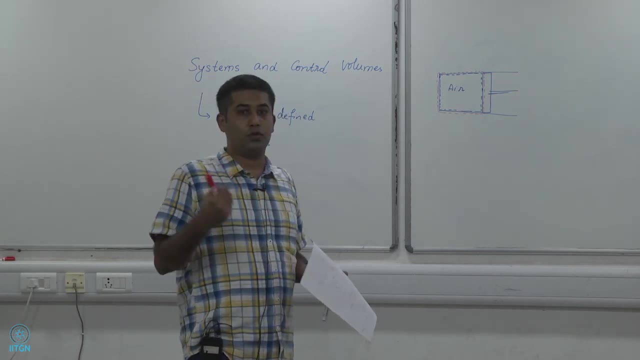 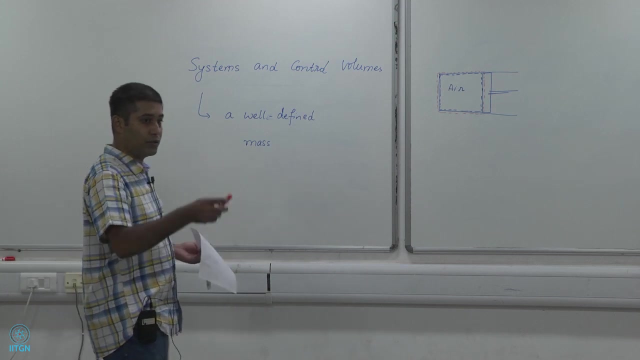 then that will not help you solve the problem. So choosing systems comes from practice, but the procedure or the attitude to first draw the system before solving a problem is what is very important. Right, You have a question? Okay, Thank you. 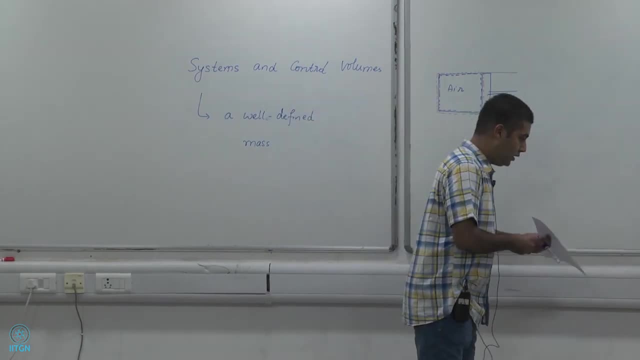 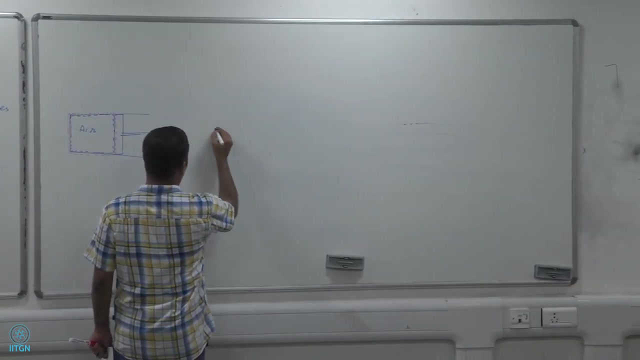 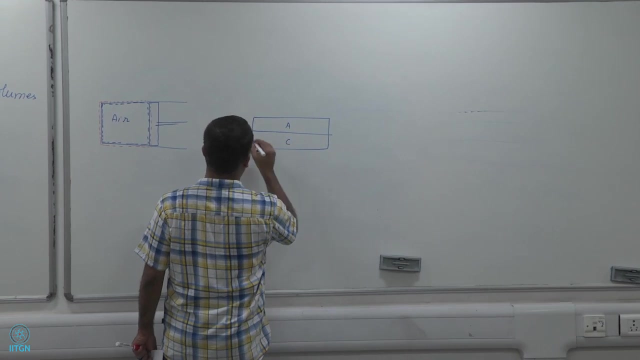 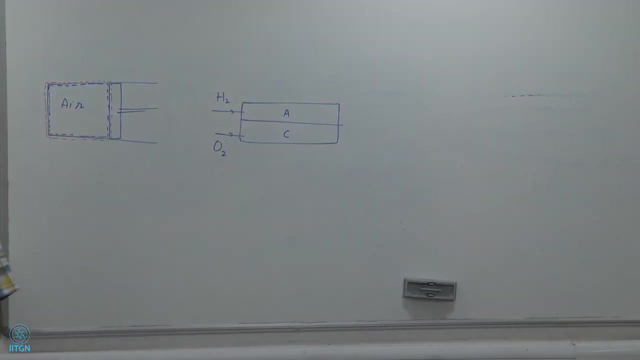 So now, what is a control volume? Control volume is a very commonly seen thing in all thermodynamics. So, for example, many of you might have heard of fuel cells. Right Now there are different kinds of fuel cells, but some of the most common type of fuel cell. 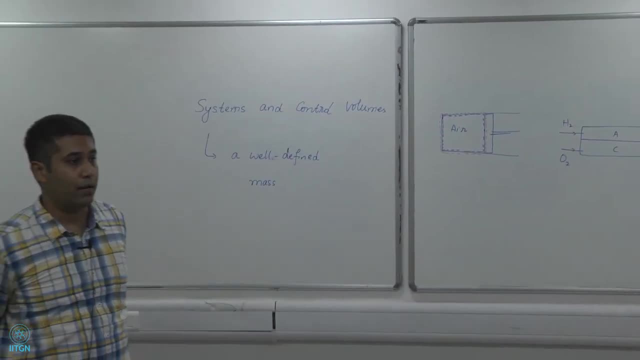 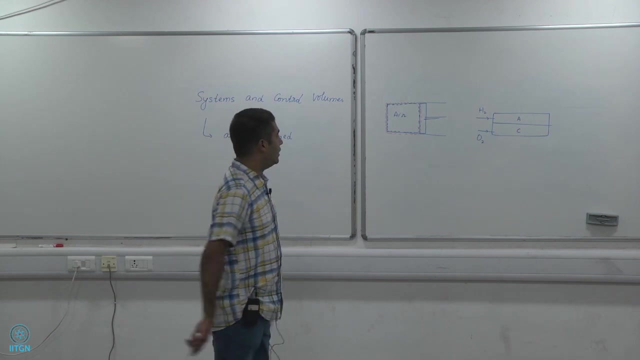 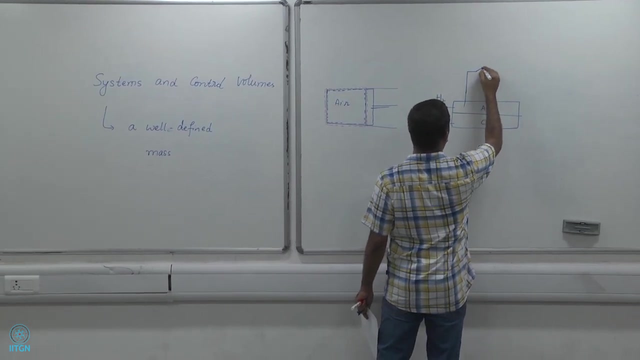 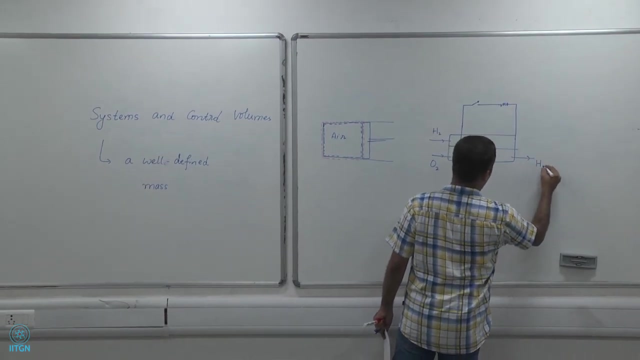 is that a device which takes in hydrogen and oxygen, and it takes in hydrogen at the anode, it takes in oxygen at the cathode and it converts the hydrogen and the oxygen to electricity. So what you get is electricity and you get some water out. 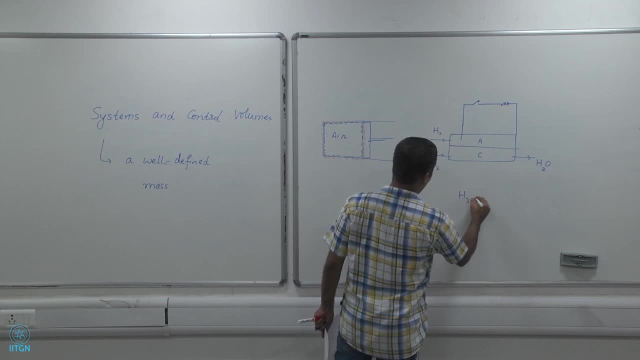 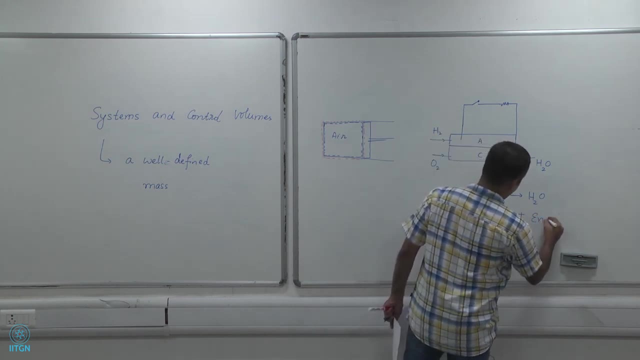 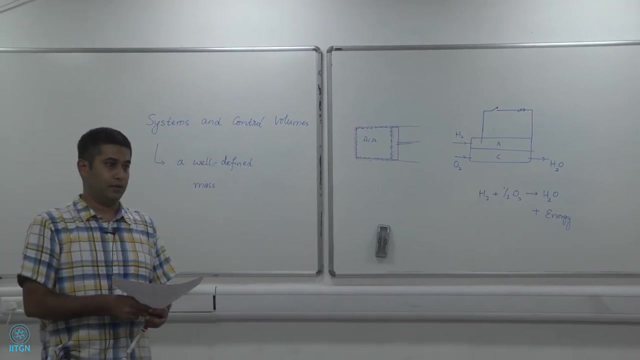 Right, And the overall reaction is H2 plus half. O2 gives H2O plus energy. Now, if you just burn it, you get thermal energy, but if you use a fuel cell, you get electrical energy. Right, You also get a little bit of thermal energy, but we will come to that later. 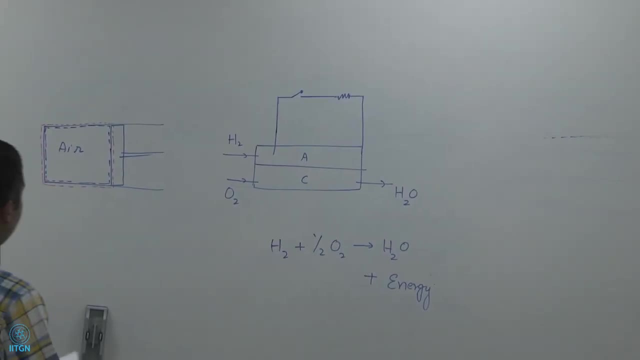 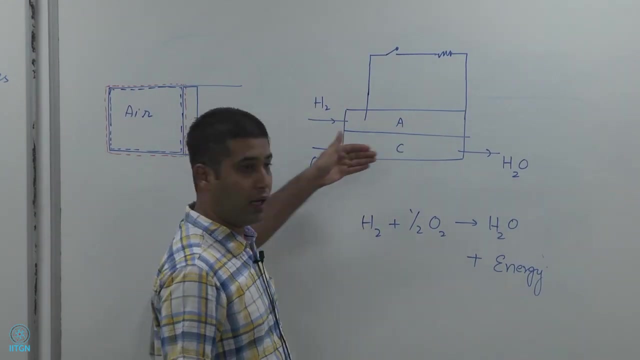 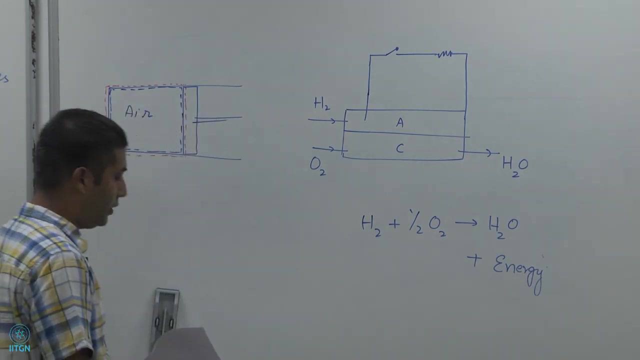 Right Now, obviously this fuel cell. If I consider that as a system, I have hydrogen entering, I have oxygen entering, I have water leaving Right, So clearly it cannot be a system. but I still can work with something called a control volume.